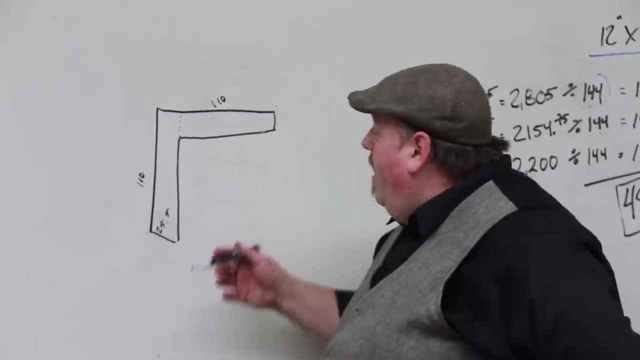 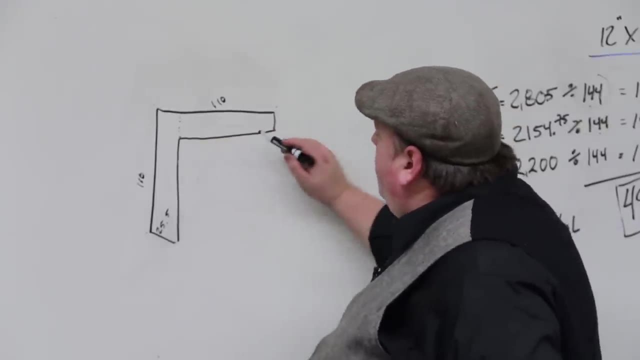 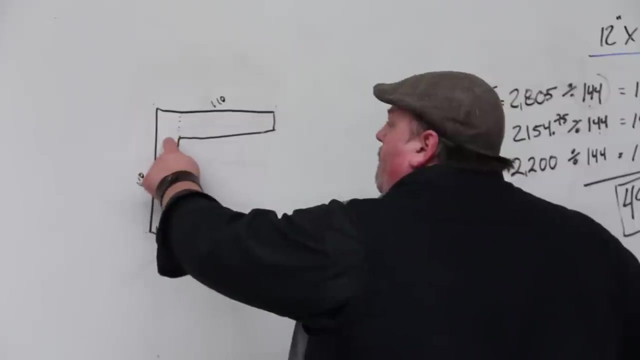 I draw a little box That is not for a seam. That is to show what box I'm measuring: Think boxes, boxes, boxes. So here's my first box. Here's my second box, but I don't want to be charged for this, so you have to subtract this number. Remember this width. 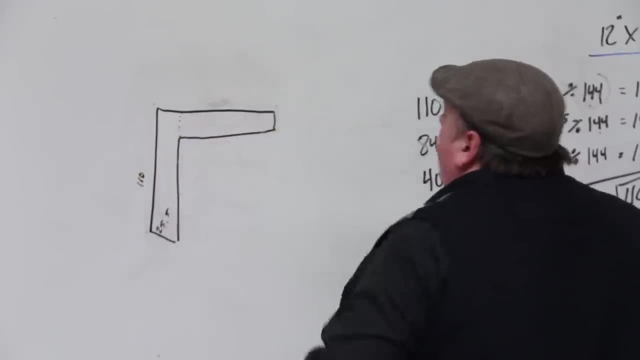 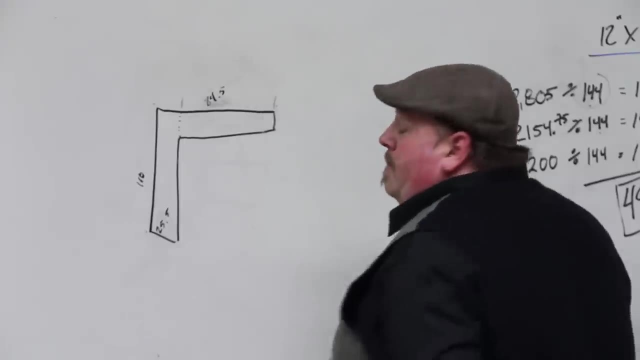 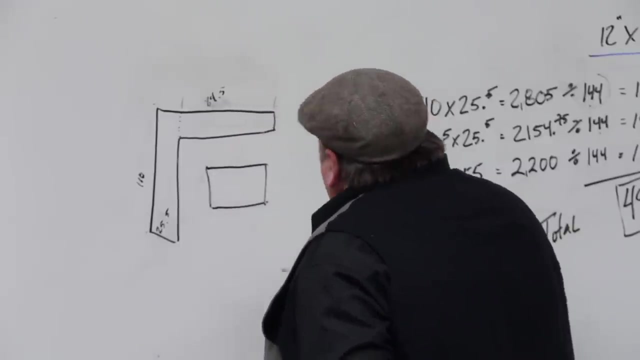 needs to come off of that number. So this really isn't 110.. This is now 84 and a half from this point to the back of the wall. okay, You also might have an island, So let's draw a little island here. Let's say that's 40 by 55, a good typical size. Let's also include 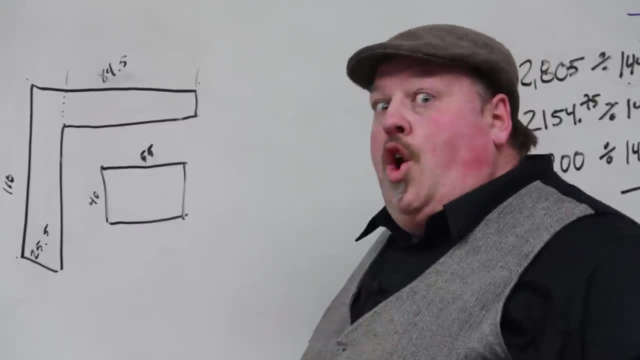 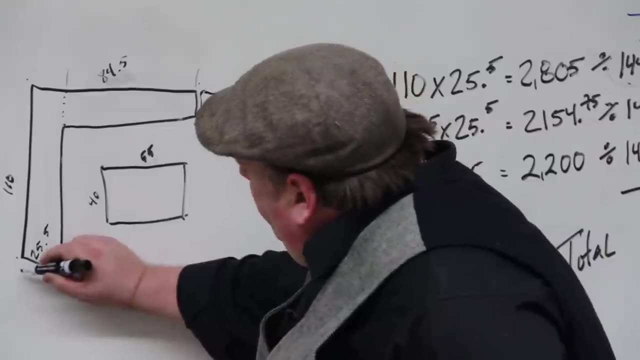 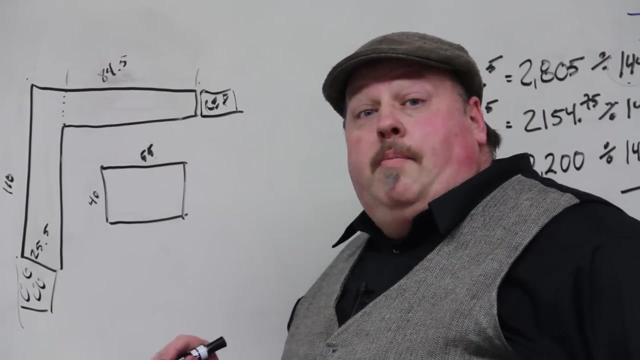 where your refrigerator and your stove might be, because we're going to want to know that down the road. So let's say: right here is your refrigerator and down here is going to be your range- Just important things that we know. Let's talk about math, shall we? Now that we've got everything squared up into boxes, let's break that down. 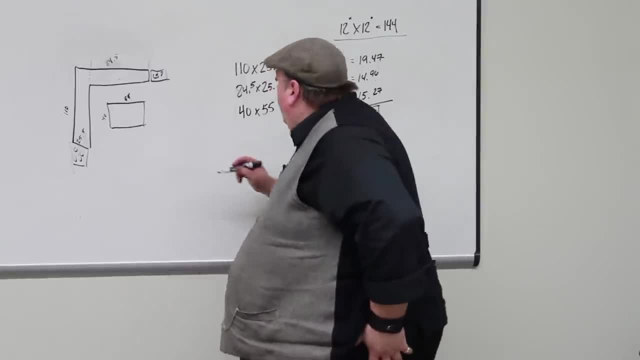 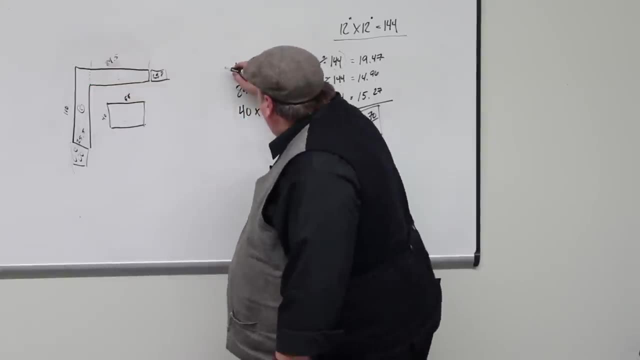 on how this is going to come out to be your square footage. okay, Now again, as we're looking at boxes, I'm going to call the first run that we put up there number 1.. So we know that box number 1 is 110 by 25.5.. Here are your inches Divided: 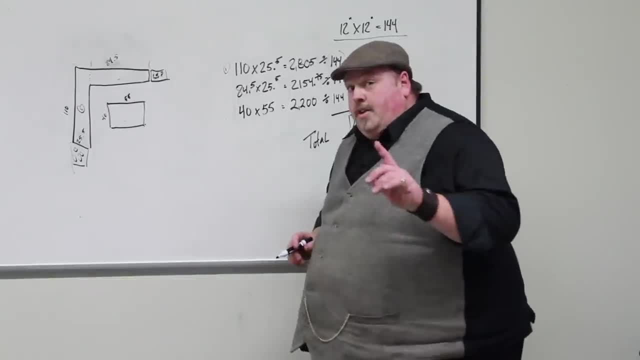 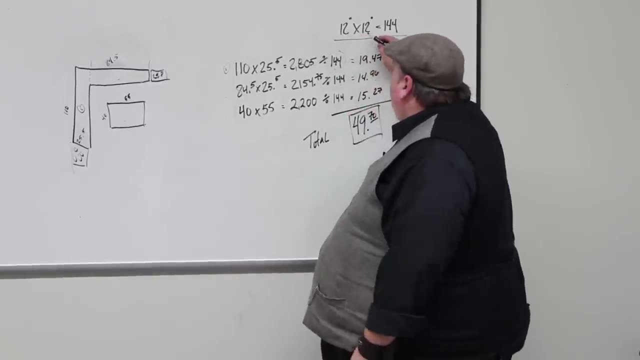 by 144 equals 1947.. Some of you want to know where do we come up with 144 and why is that a magic number? The reason being is 12 inches by 12 inches equals 144.. There creates our square foot equation. So that's our magic number. And so, as you see, with box number, 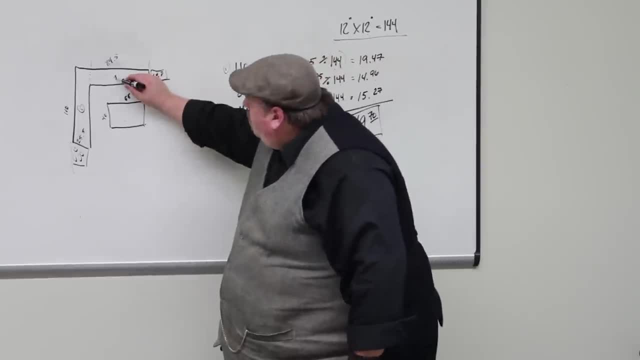 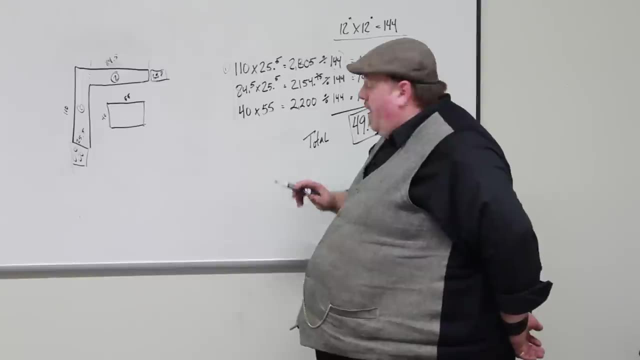 1,, we're at 1947.. Box number 2, which I've subtracted the width of the counter. that gives us 84.5 times 25.5.. Again, your inches divided by 144.. Here's your magic number. 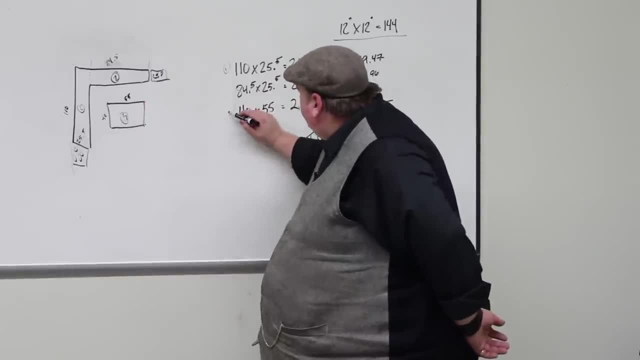 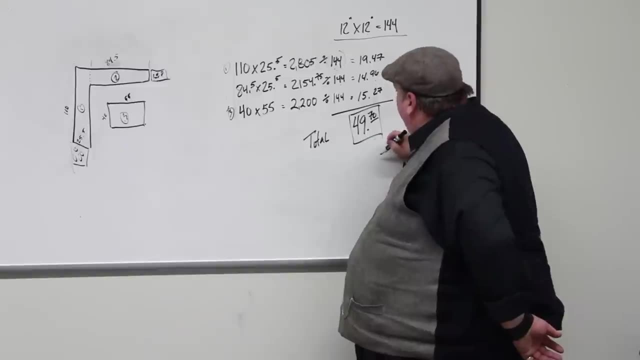 Let's say, box number 3 is the island That's right here. 40 by 55.. Here's your inches: 15.27, giving you a grand total of 49.70.. Basically, a 50 square foot square foot. 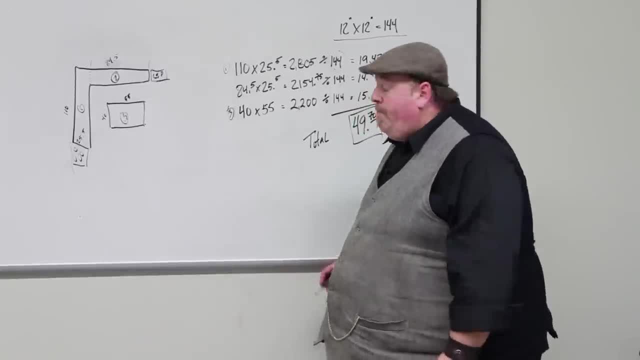 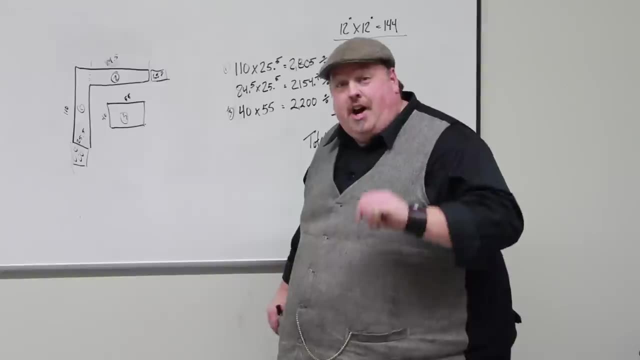 Which is what a lot of our clients have Very common. So very simple folks, You know the formula, But you may be saying my shape of kitchen is not here. Let's talk about some other shapes and this will make more sense. 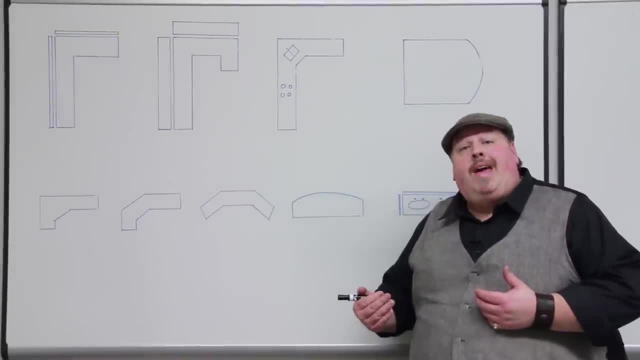 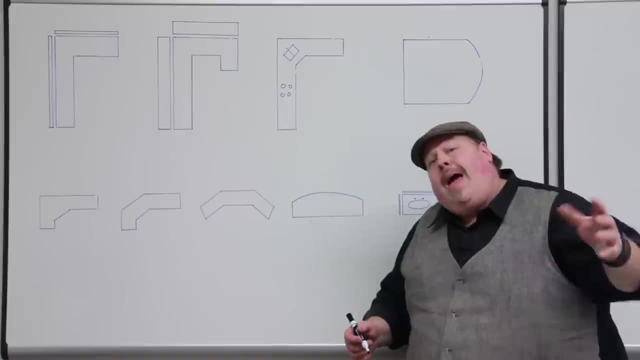 So many of you, when you're calling, are concerned because you may have other shapes that don't fit in what we've shown you. Maybe you don't have an L shape, Maybe you have a curved piece or some angles. Now we deal with that every day. It's quite simple. Let's start with an. 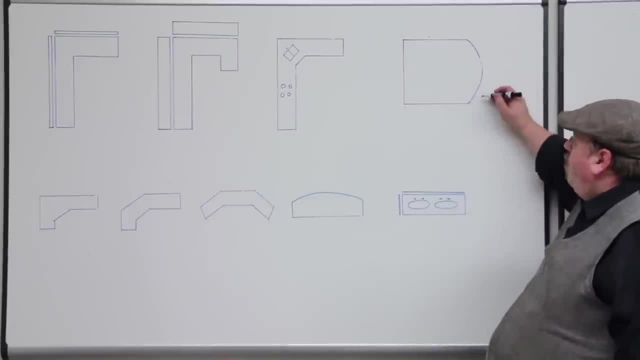 island. Many folks want a radius corner on your island. We love to do that. It looks very tailored To calculate that. find the widest spot on the island in the center, and then basically we're going to draw this imaginary line out and now you have a rectangle again. So you 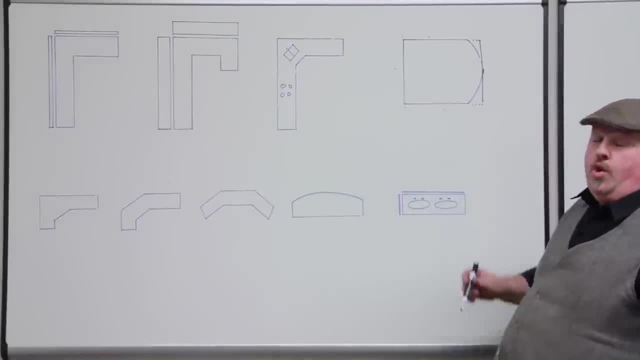 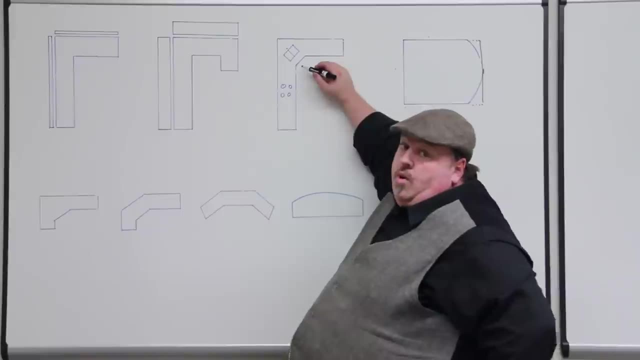 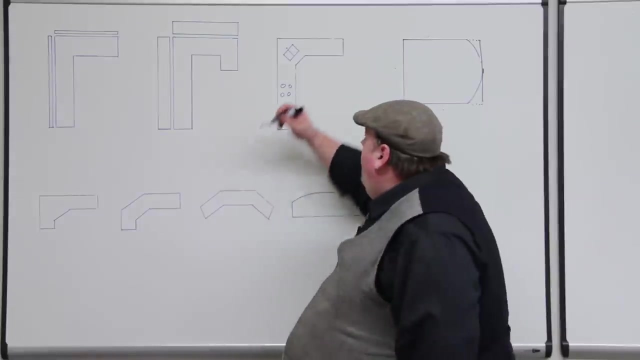 times width, times length, divided by 144, and you're going to have your number. Very simple. Now, many people get a little confused when you have this angle in the corner with a sink kind of facing out Again. it's all about boxes, Think boxes. 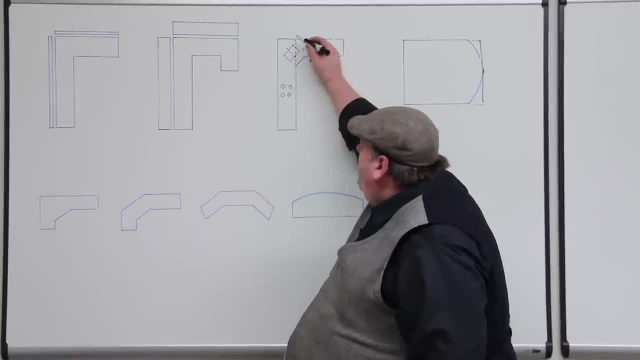 Take the long side and oh, remember how I told you. I just draw a little line. That's not a seam, It's just how I measure. So this is going to be one box, and now I do the same here. This is going to be a box and to be safe anytime, you have this triangle here. 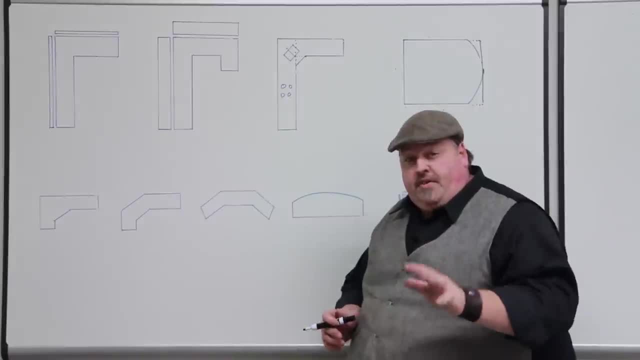 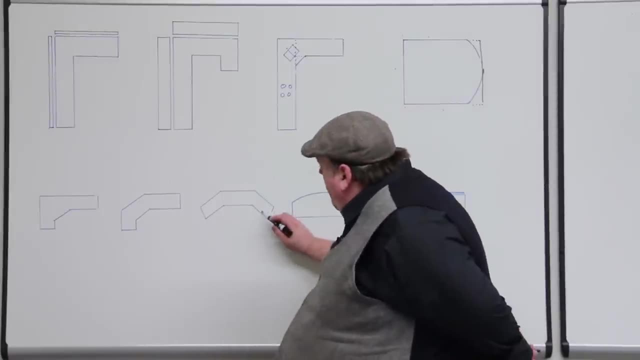 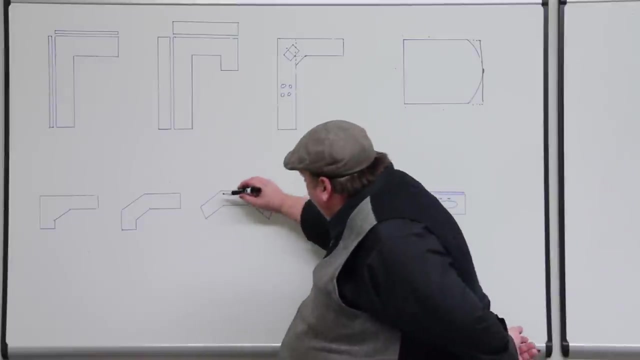 figure that's going to be about 1.5 square feet, So one and a half square feet. You add these and you're done Something a little more complicated. A lot of you have these three winged peninsulas or islands- Think boxes, Real simple. This is a box here. This. 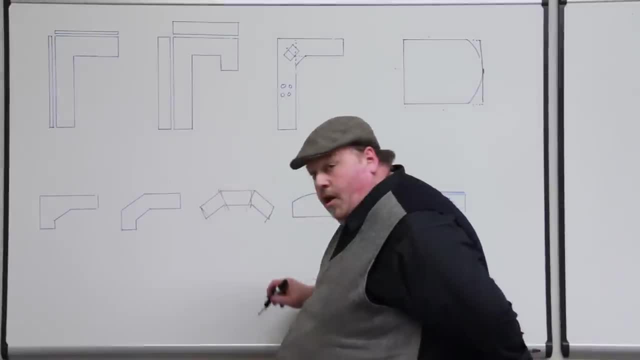 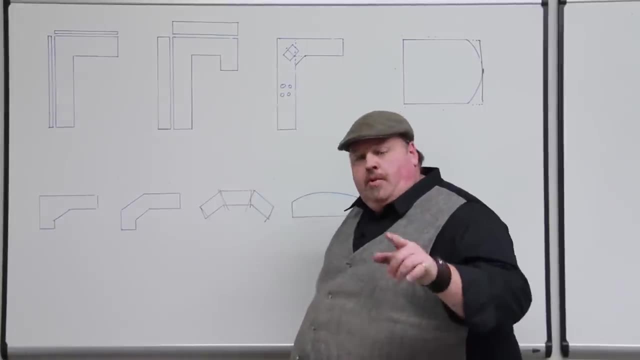 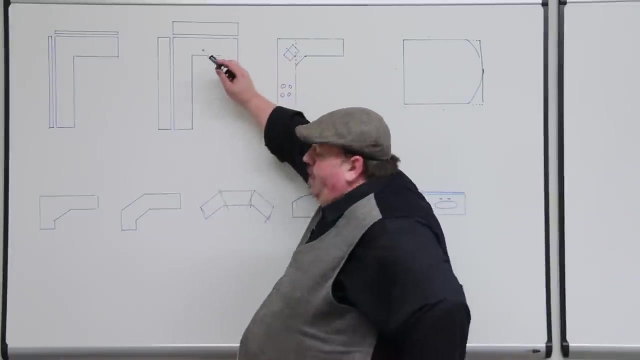 is a box here. This is a box here. There's going to be some overlap, but once your template is remeasured, after it's made, your numbers will be recalculated and most likely, this number will go down. Backsplash: Very popular. A lot of folks want full backsplash. Very simple, Same formula.